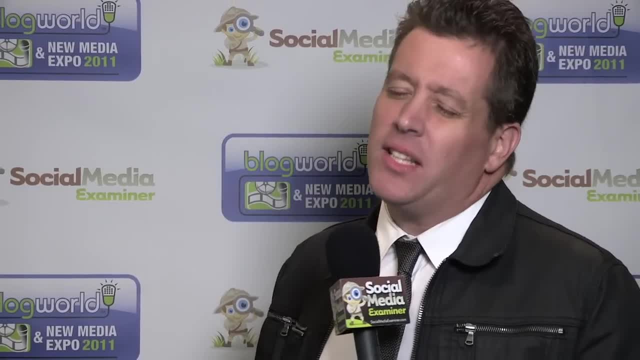 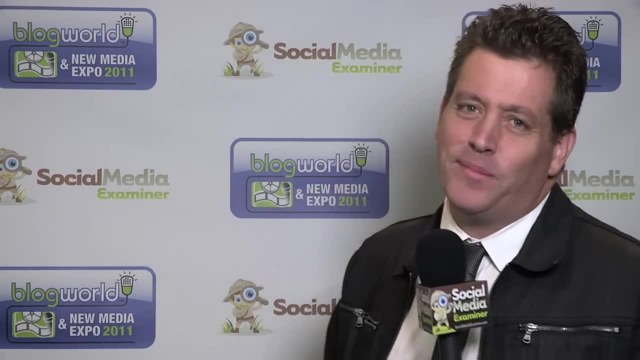 Had I built that No7, would have been there. So I think it's. you know, it's what's the classic joke, The hardest part about being a comedian: Timing: Yeah, There you go. So yeah, Awesome. Can you share some examples? 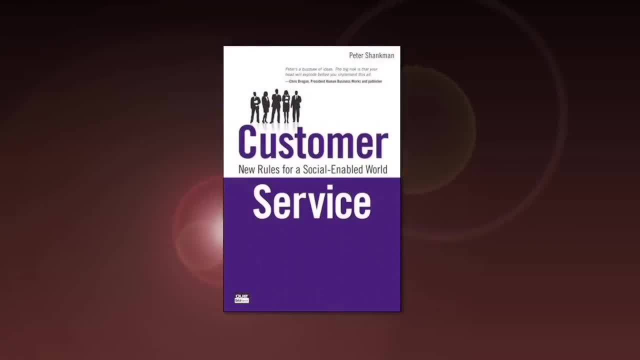 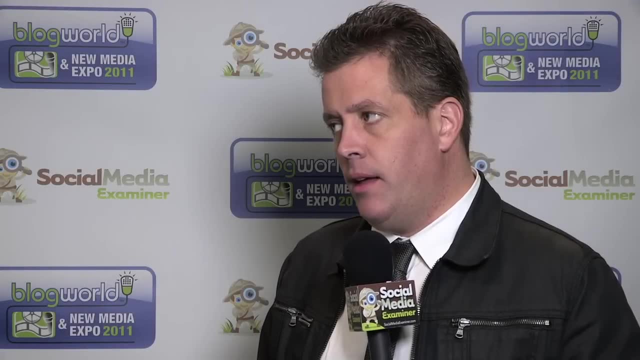 Oh, by the way, I also forgot to mention your book. You're the author of Customer Service: New Rules for a Social Media World, So I want to talk to you a little bit about some. what are some businesses that are doing customer service well? 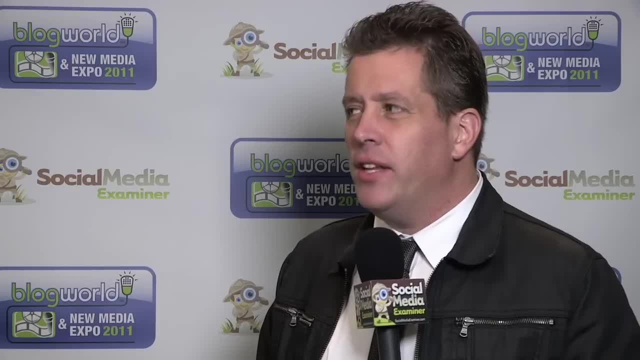 United, United Airlines is doing a great job. What are they doing well With the merger in Continental? they've really been out in front of the merger talking to people, kind of calming their fears- Oh, am I going to lose my status? 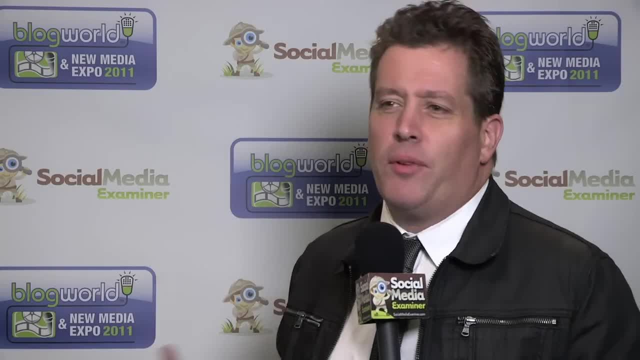 Am I going to lose this? and that They've really done a great job with keeping people aware of what's going on with the brand and, when they have problems, responding almost immediately. back On the flip side, there are sites out there that say: 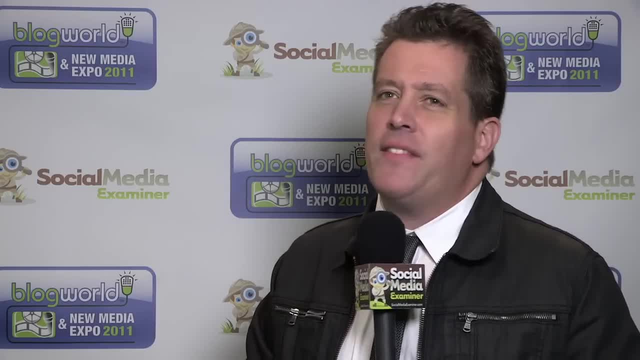 hey, you know. thanks for being on our social media page. Unfortunately, we don't have the time to answer you here. Please send us an email, please call us, I'm like. well, what the hell do you have a social media page for? 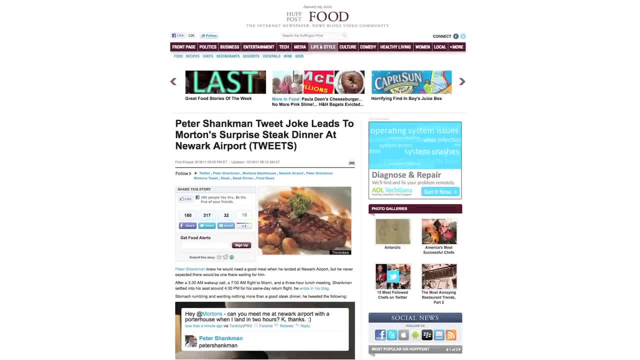 You know there are other companies out there. Gotta mention Morton's. I tweeted out as a joke last summer. this past summer I said: hey, Morton's, I'm starving. Why don't you meet me at the airport after my flight with a porterhouse? 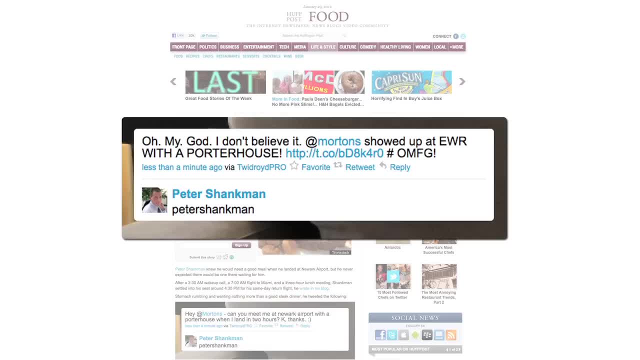 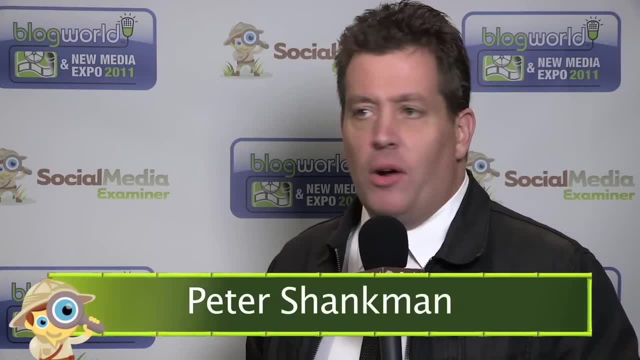 And someone saw it on Twitter: Morton's showed up with a porterhouse, Morton Steak showed up with a porterhouse at the airport. I mean it's. those are the kind of things. How did that impact you as a customer? I will go out of my way to go. 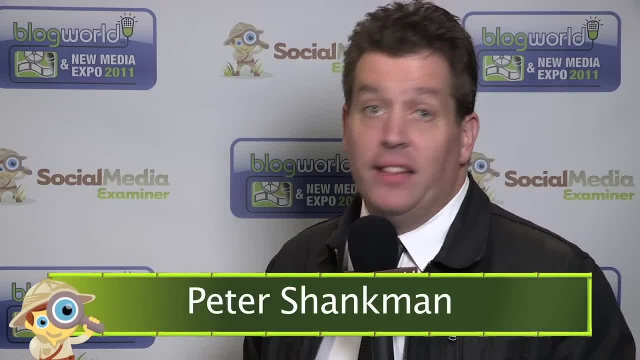 I was supposed to go to another steakhouse last night. I realized there's a Morton's downtown Change of reservation right on the fly. I love them. now they have won me for life. So what's the message to businesses here? Listen four times as much as you talk. 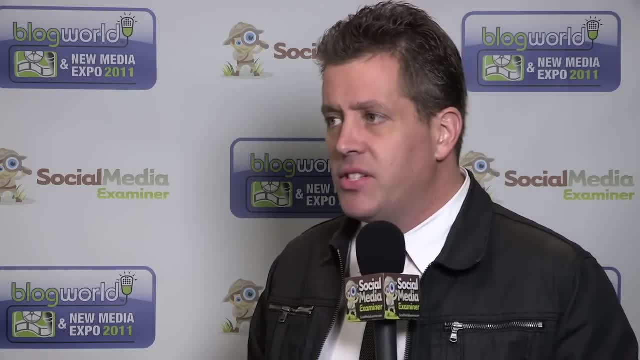 So how do they go about doing that? Very simple: you do searches for your name. you see what other people are talking about. listen to your competitors, search for your name, search for misspellings of your name. You know, be out there, see what people are talking about. 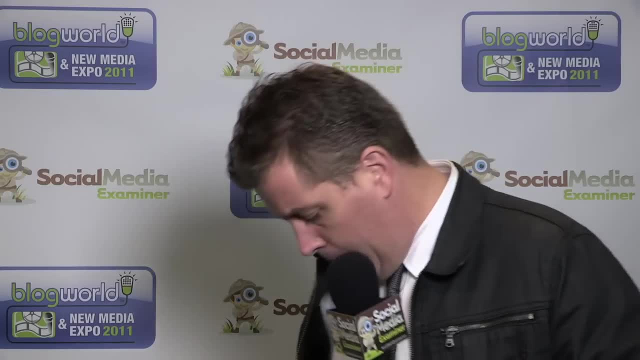 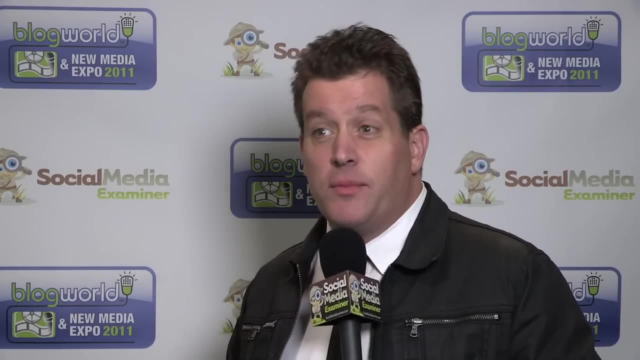 and then get in front of the issues. If there are problems, deal with them. So, speaking about problems, how do businesses deal with upset customers? What's some of your advice about that? I wrote about this in the book. The thing you want to do, break down the type of customer. 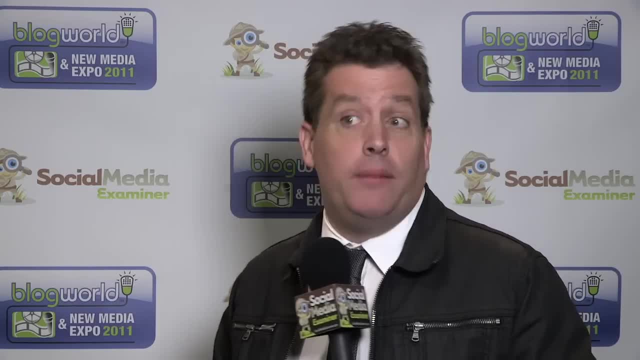 Is it a customer who's never complained before and you look them up and you realize they've spent thousands. You've got a problem. deal with it immediately. Or is it a customer who likes to hear his own voice, likes to complain a lot and has three followers? 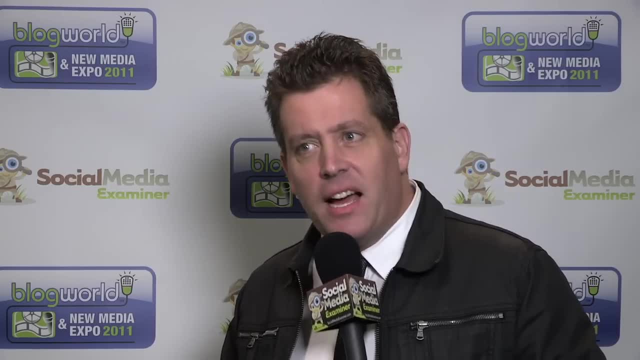 Chances are they've done this before. Placate them, you know. sorry, you had a bad time. next time you're here, come in and we'll give you a free drink, whatever the case may be. But the worst thing, the only thing you cannot do. 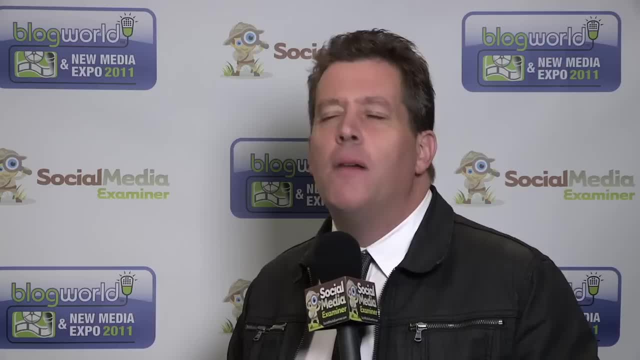 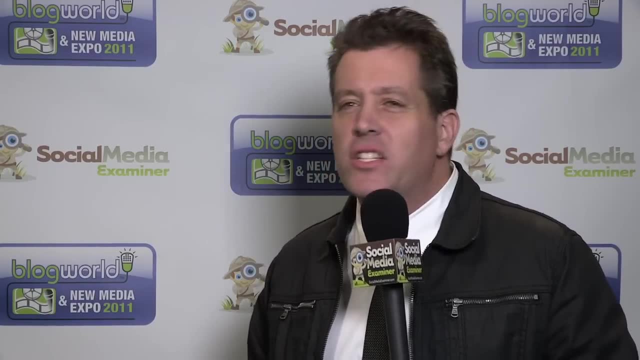 is ignore them. you have to focus on them, Even just in the most minor way. but focus on the customer. Everyone loves to know that they were heard and even if you don't fix the problem entirely, at least make sure they know they've been heard. 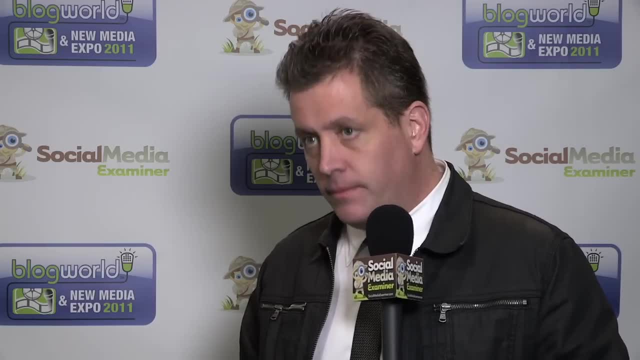 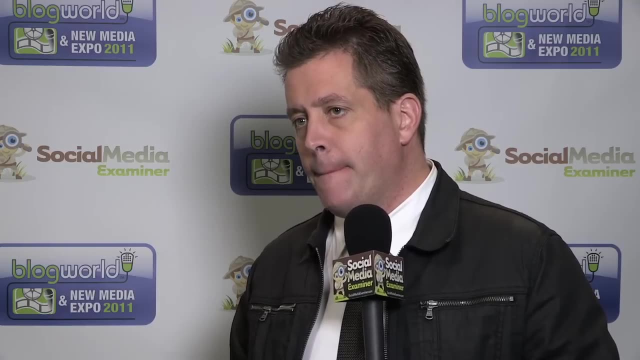 You brought up an interesting point here about look up the customer. Are businesses actually savvy enough today to actually look, say hey, is this person super influential to us? They don't even need to be super influential. that's why I think the cloud score is BS, you know. 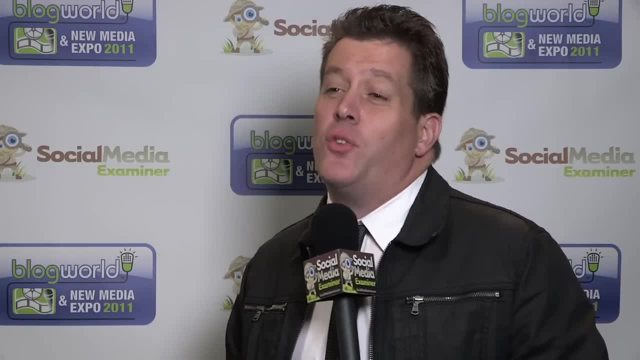 Yeah, Talk to the customer. ask the customer. if a customer comes to the wine store and asks for a very specific brand of red- I know he's smart about red wines- Right, That to me is an influential customer, Gotcha. 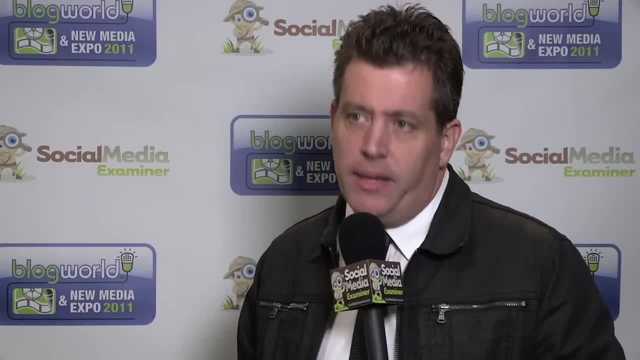 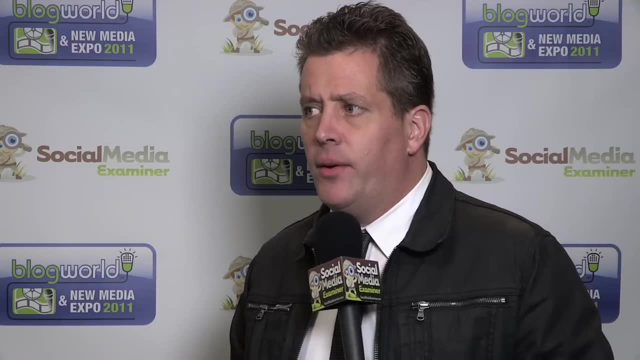 You know, it's not about a score. it's about knowing your audience and knowing what you want your audience to be Right, Very cool. How has social media impacted public relations in your opinion? Hey, it's changed it drastically. You know, everyone can be a journalist now. 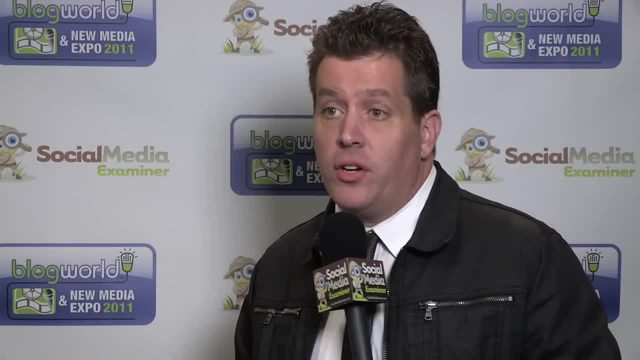 everyone can be a reporter. stories can break online. they don't need to necessarily go through journalists. but, that being said, journalists still have a lot of power and you do need to respect that. And you know you have the ability now. 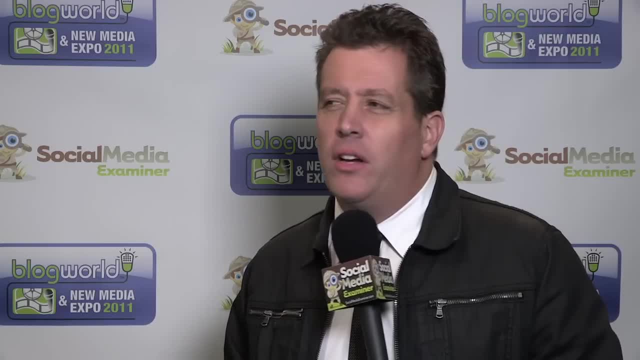 there is no excuse for pitching off topic anymore. You have the ability to look up any journalist, see what they're tweeting, see what they're talking about, to then pitch them. something that doesn't isn't something they're doing is just a complete 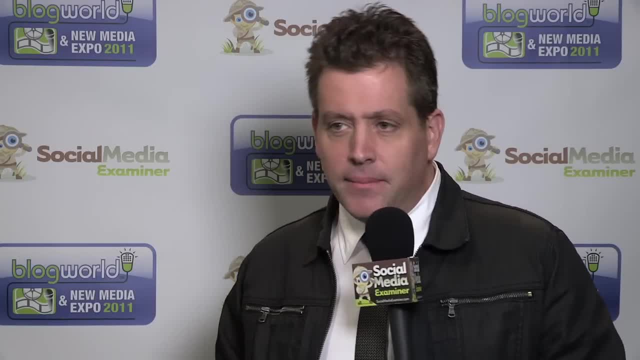 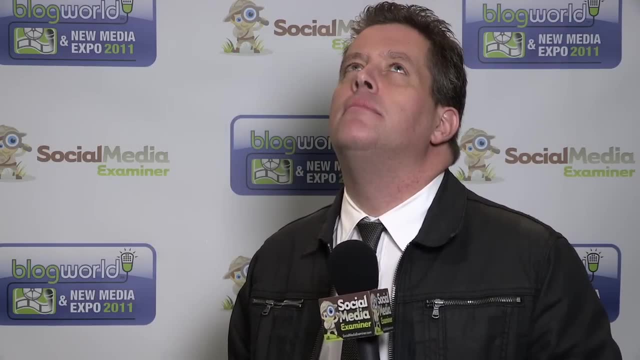 and utter waste, so you should be shot for it. Speaking of being shot, Peter, what is in your mind the thing that businesses are doing wrong? that just gets you crazy Not taking the time to learn about their customer. Again, I got a letter from a car dealer. 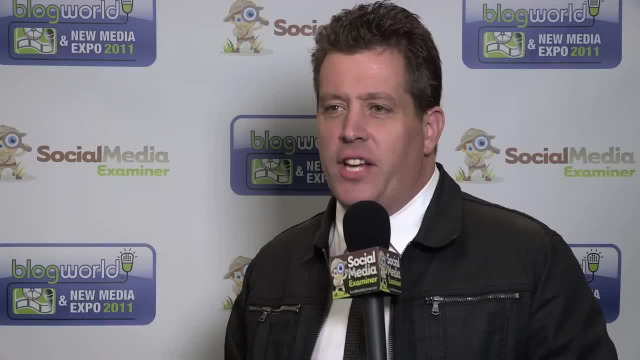 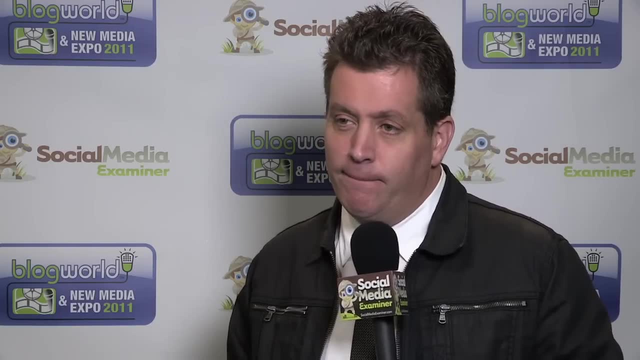 I was returning my lease on a car dealership and the letter said: Dear Mr or Mrs Peter Shankman, I'm like really, Really, Was that freaking hard? Yeah, Okay, how long has it been since you've been? 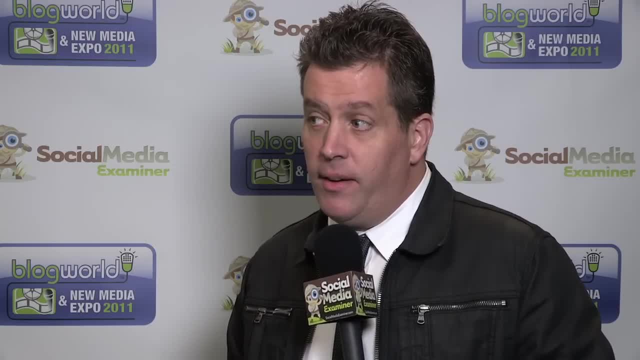 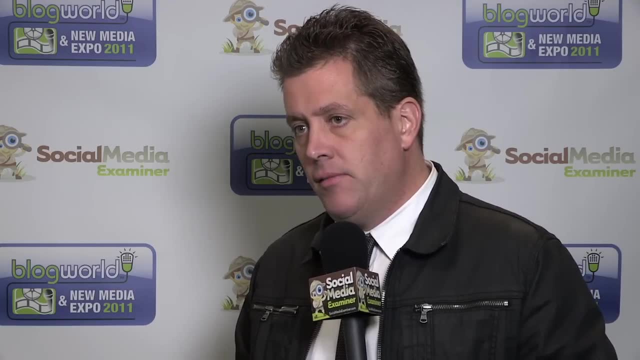 when did you start HARO? what year was it? HARO started in November of 2007, and it was acquired in June of 2010.. Okay, so, since November of 2007 until now, there's been a lot of things changing. 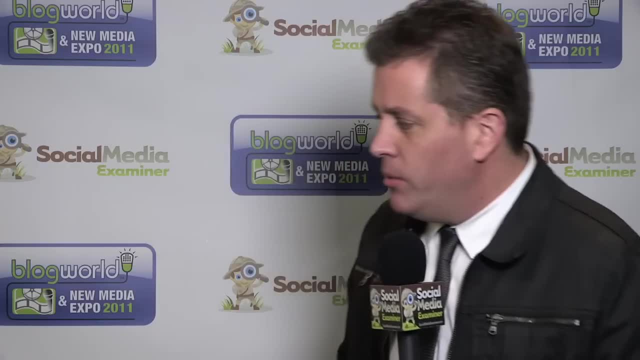 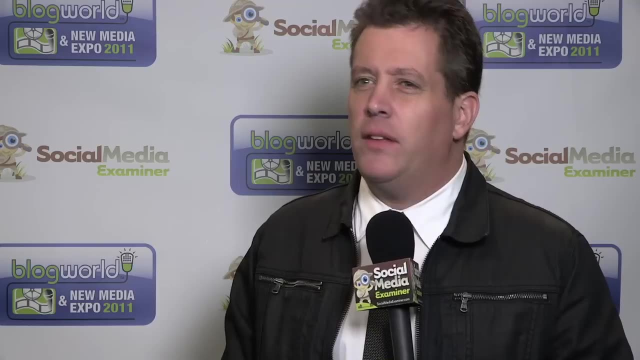 What's your perception of where things are going? I think we're moving more towards a world where it's about relevance. You know, from the friends you hang out with to the companies you do business with, it's more about relevance and the more relevant they are to you. 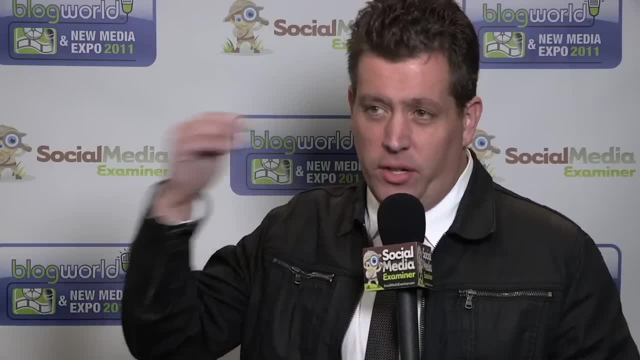 the more they'll show up in your stream, the more you'll see them in your profiles, the more you'll interact with them. When they stop being relevant to you, they'll just fade away. I think the concept of friending and unfriending. 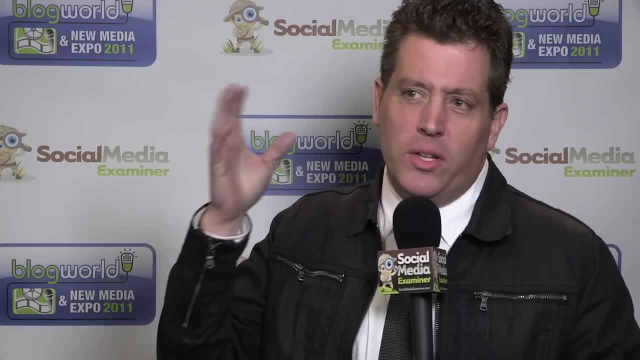 is gonna go away. If we're friends and we hang out, we'll be friends online. We're going through the digital world. Once we start not hanging out anymore, the system will know that We won't check in together, we won't be at parties together. 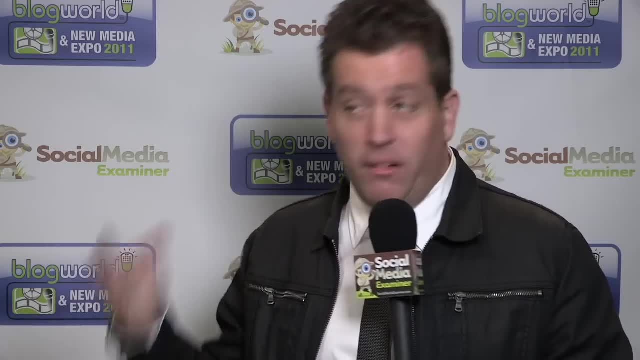 we won't have our photos together, we won't be tagged together, and the system will get smarter and learn that and just slowly stop the friendship process. So does that mean- It's like real life basically? So you see that. 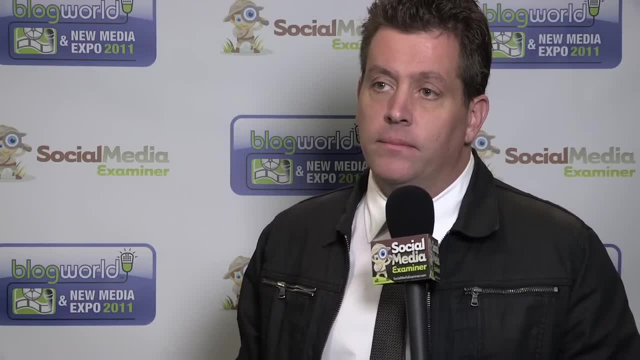 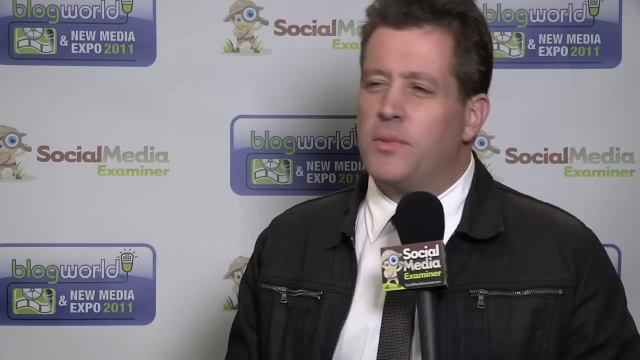 almost like what Google Plus is doing with circles. you see some sort of microcosms essentially evolving in the relationships between people. I think we're moving back to the concept of a village. You know, in the 50s the husbands would go to work. 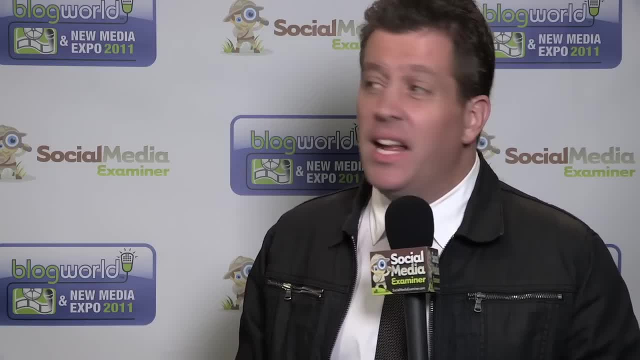 and the wives would sit there in a sewing circle and they'd talk about where to shop for meats and where to do all that. It went away with two families, two parents working and two income families and things like that. We're seeing that come back thanks to social. 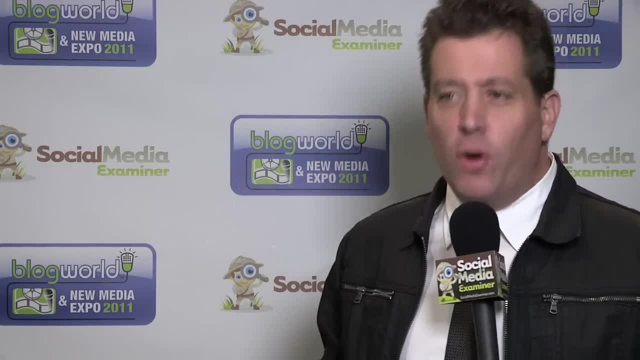 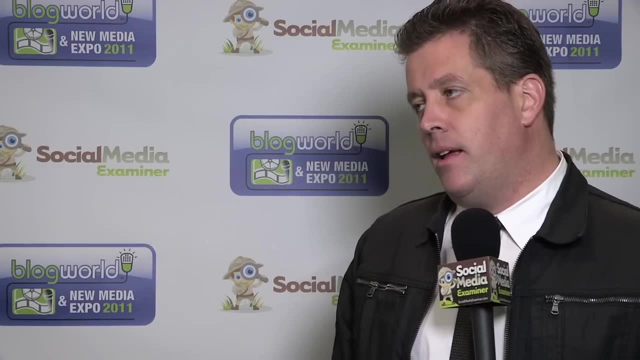 and thanks to the web, where people can say, hey, I need to get the best cut of meat. What do my New York friends think? And 10 people tell you, Peter, what's coming next from you. Is there anything special you're working on? 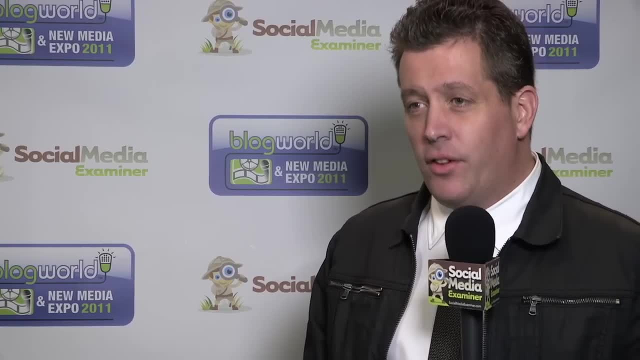 that you can share. I have a couple of different ideas. I'm working on something for TV, Oh really, I have a third book that I'm working on. So I have a lot of fingers and a lot of pies and I'm just having a friggin' blast. 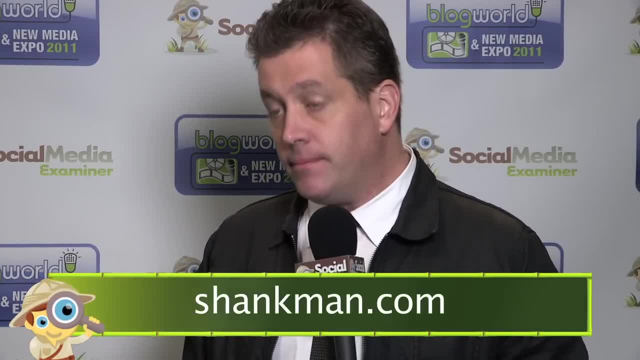 That's the most important thing: I'm having so much fun. If people want to learn more about you and about your book, where would you send them? Best bet is shankmancom. My entire life is on shankmancom. 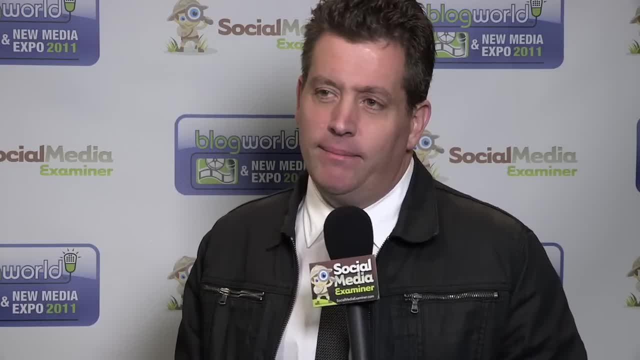 On Twitter, I'm at Peter Shankman And, yeah, you can find me pretty much anywhere. Peter Shankman, thank you very much for your time today. Thank you.